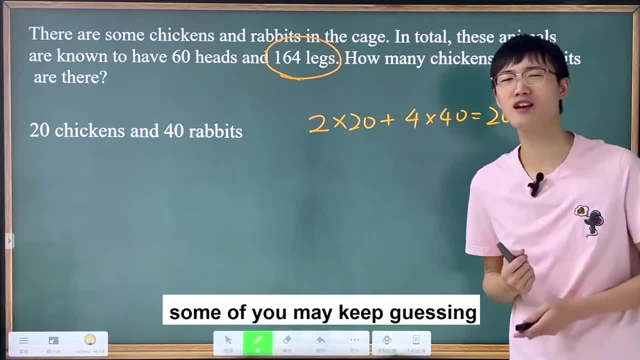 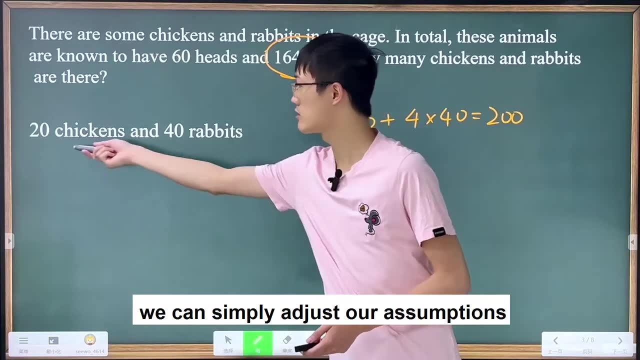 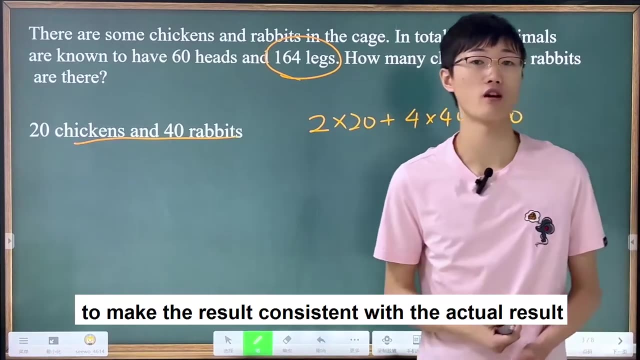 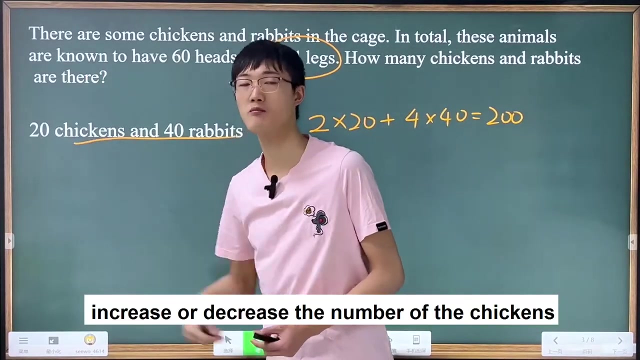 right answer. Some of you may keep guessing, but that would take a lot of time. We can simply adjust our assumptions to make the result consistent with the actual result, But we don't know if we should increase or decrease the number of the chickens. So how? 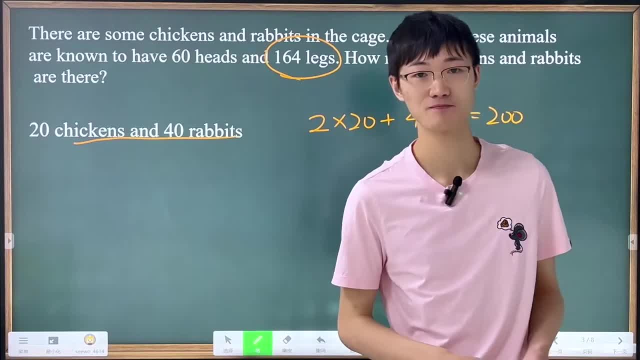 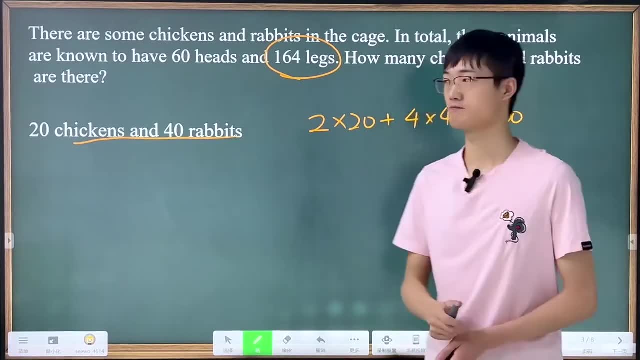 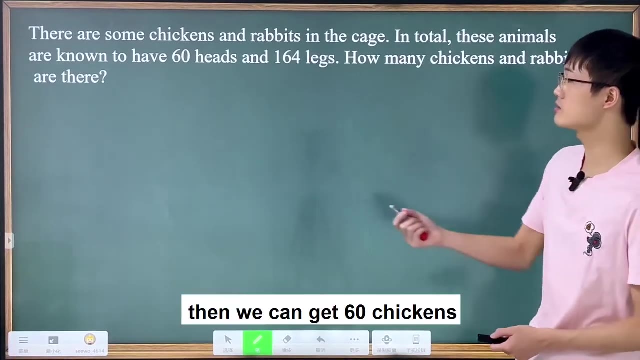 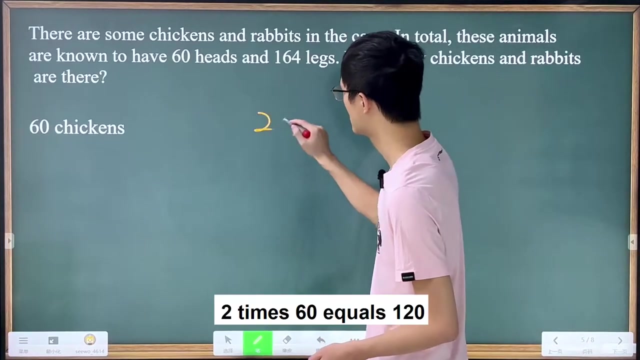 should we assume the number of chickens? Consider that, Yes, Consider the extreme situation. Let's see, We can suppose that all the animals are chickens. Then we can get 60 chickens. And how about the legs? Two times 60 equals 120.. 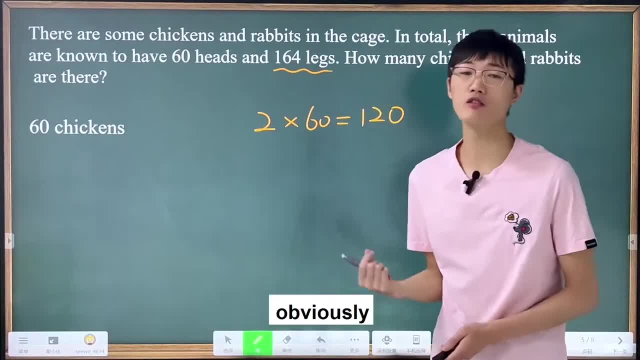 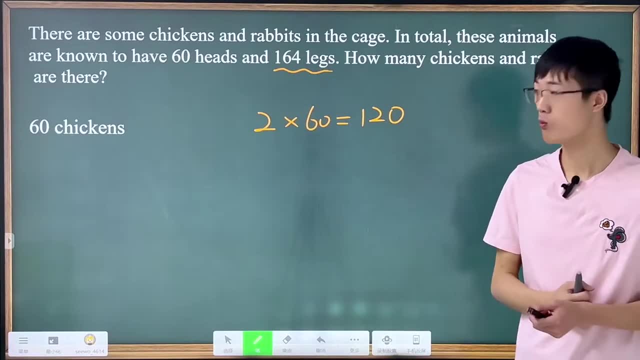 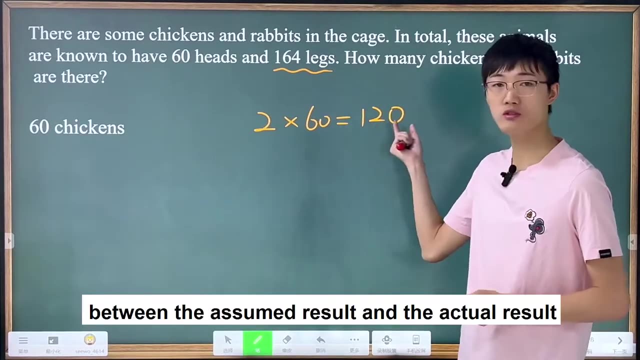 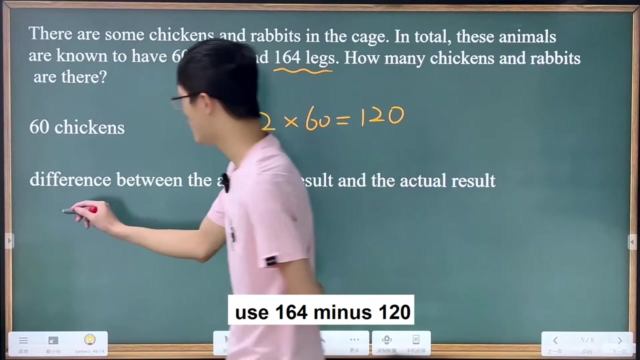 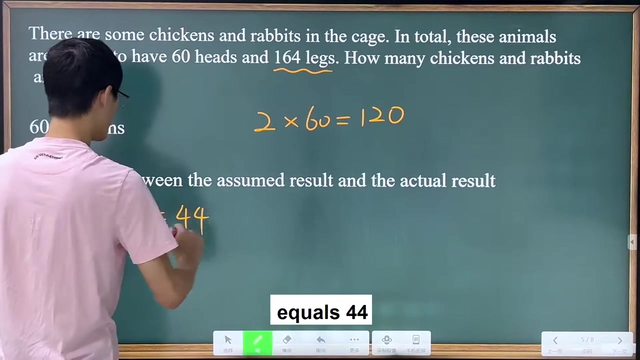 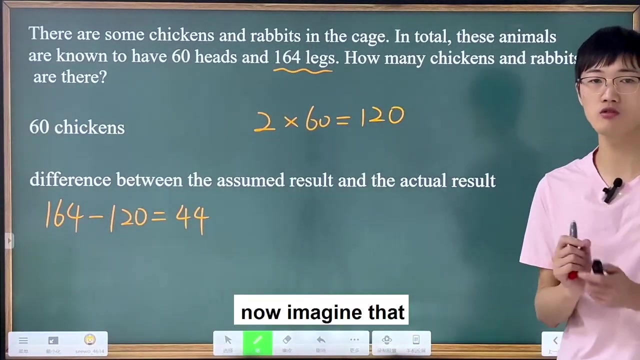 Obviously it is also not the right answer, But it's very useful. Let's see. We can calculate the difference between the assumed result and the actual result. Use 164 minus 120 equals 44.. 44 legs, Then we can imagine that there are 60. 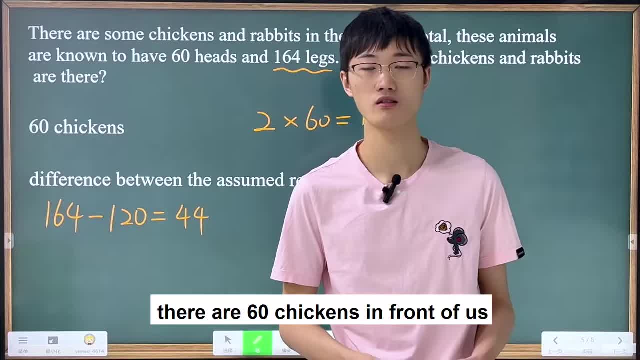 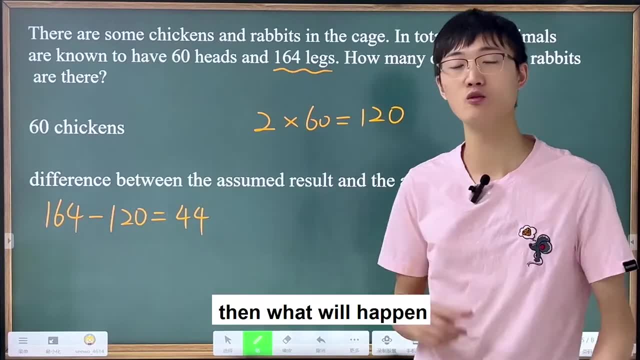 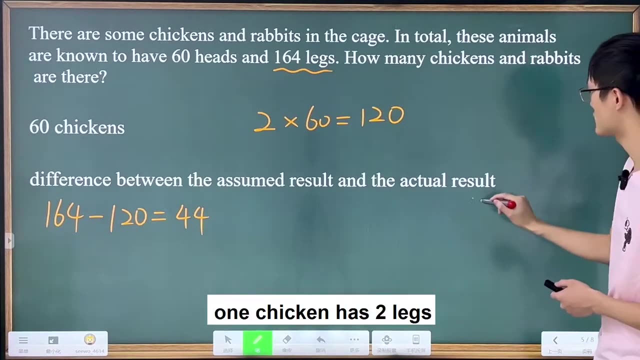 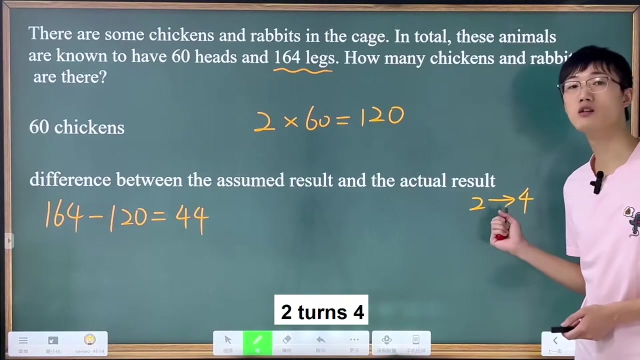 chickens in front of us, Then we replace one chicken with one rabbit, Then what will happen? Let's see: One chicken has two legs, while one rabbit has four legs, So 2 turns 4.. The number of the legs of all the animals includes ahasص below x. 4. alert estoy de. ocho s shoutico x trick altois. The number of legs is called 4 times 100. Which delta does the grau, Celsius, uh, ego and pareto of all the four legs times one, 3 times 20 plus two? In such a case we have: 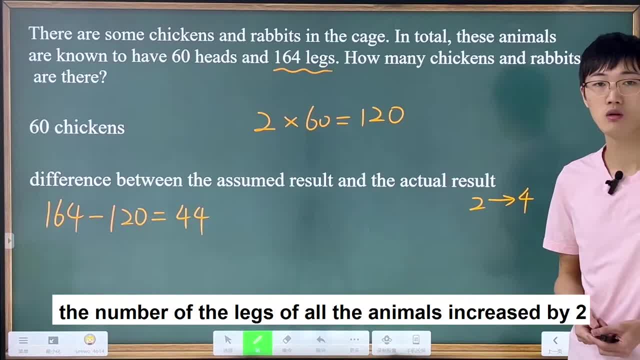 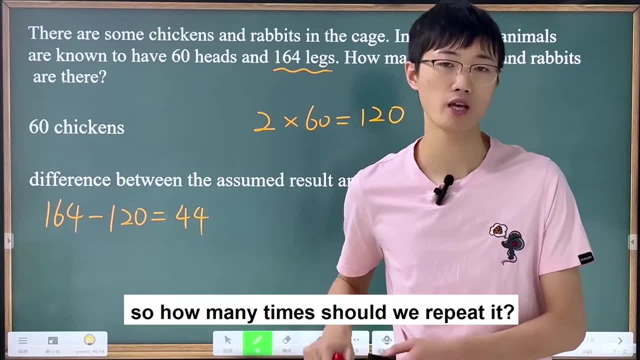 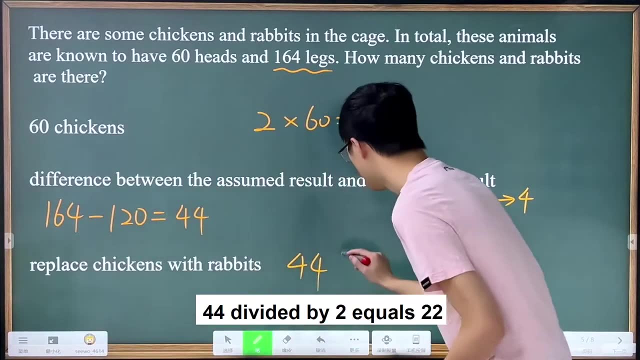 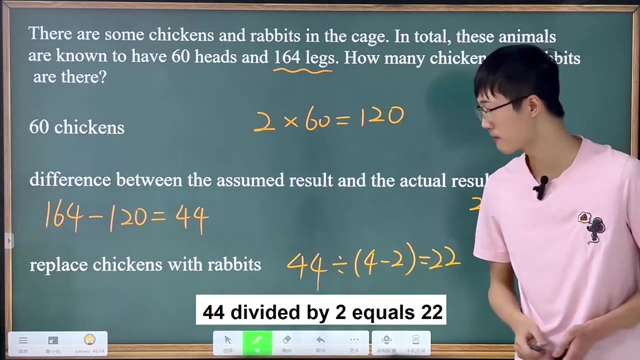 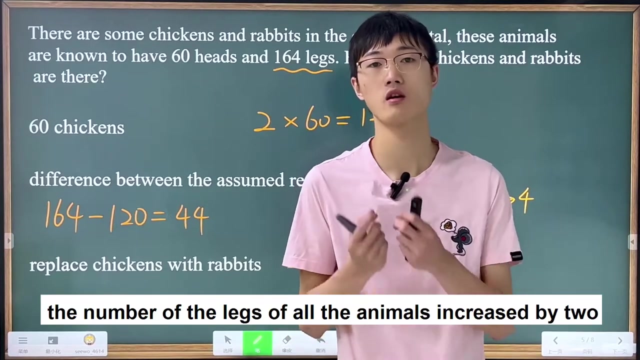 increased by 2.. But our target is 44, so how many times should we repeat it? Yes, 44 divided by 2 equals 22.. That means we replace one chicken with one rabbit. The number of legs of all the animals increases by 2.. Then this progress would. 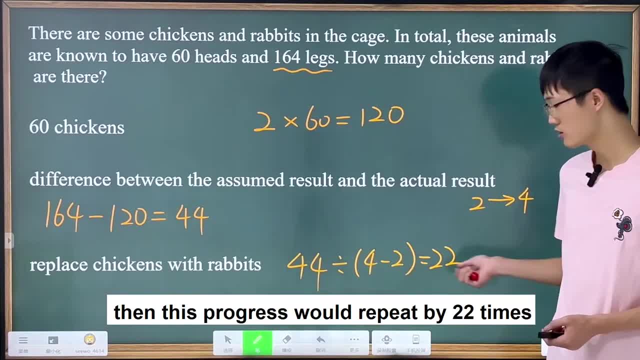 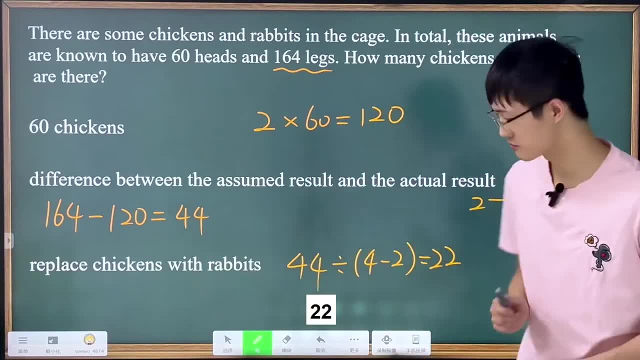 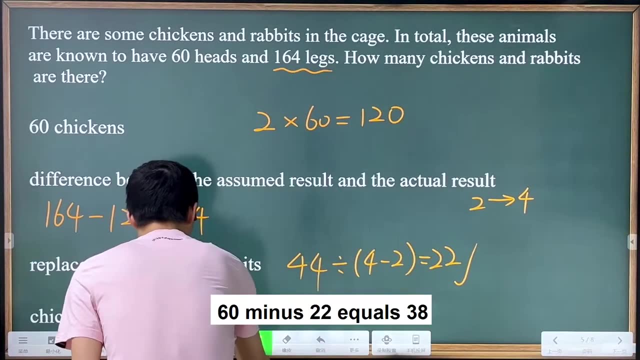 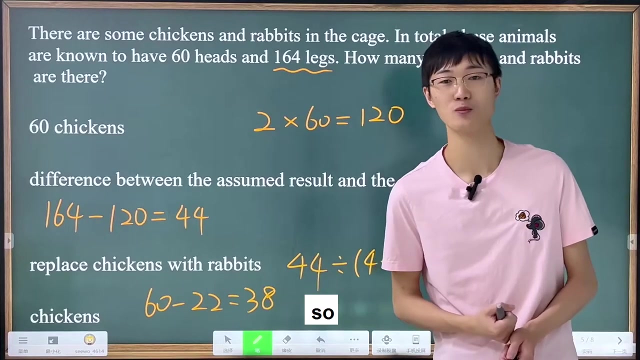 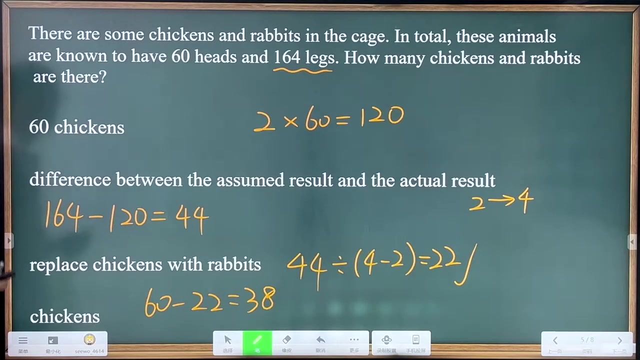 be repeated by 22 times. Then how many rabbits are there in the cage? Yes, 22.. Now how about chickens? 16 minus 22 equals 38.. Finally, we solve it. So let's see our conclusion. A chicken and a rabbit question. How to solve it? First of all, we may suppose that all the animals 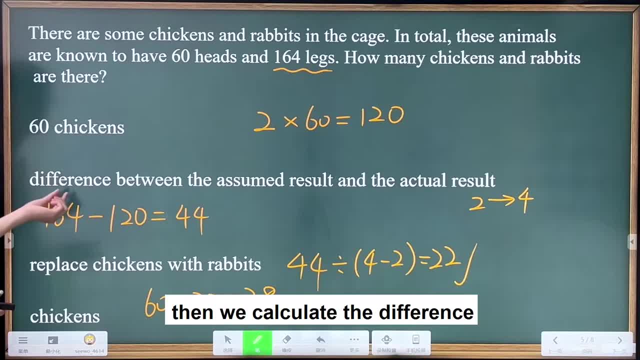 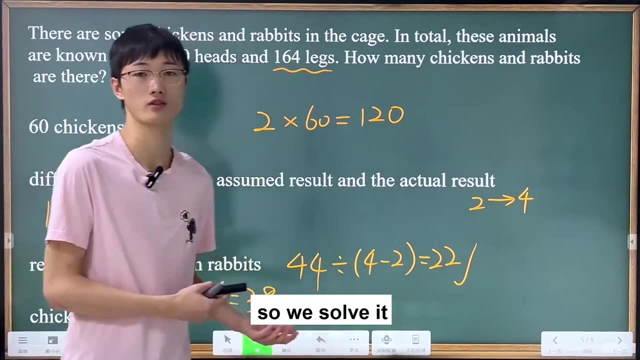 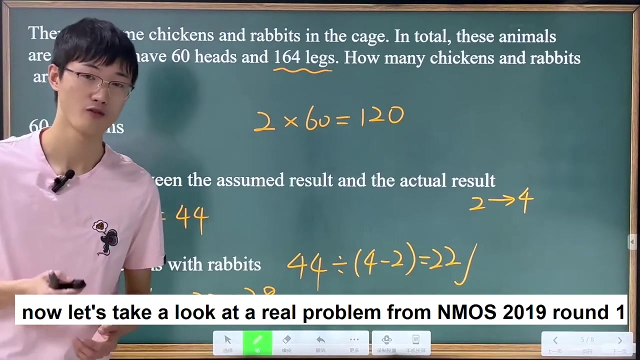 are chickens, Then we calculate the difference between the assumed result and the actual result. Thirdly, we replace chickens with rabbits. Then we get the number of rabbits. So we solve it. Okay, have you got it? Now let's take a look at a real problem from NMOS 2019, round 1.. 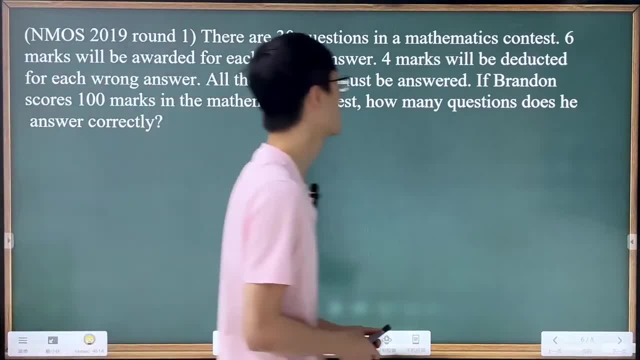 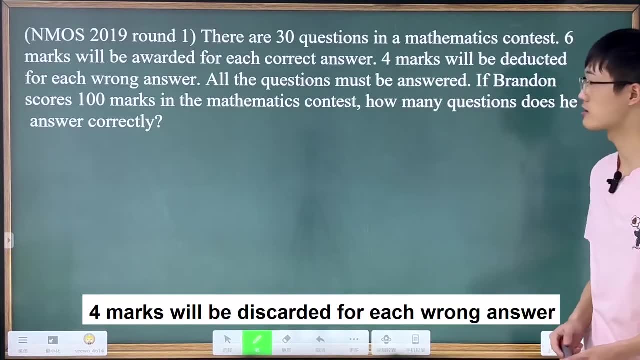 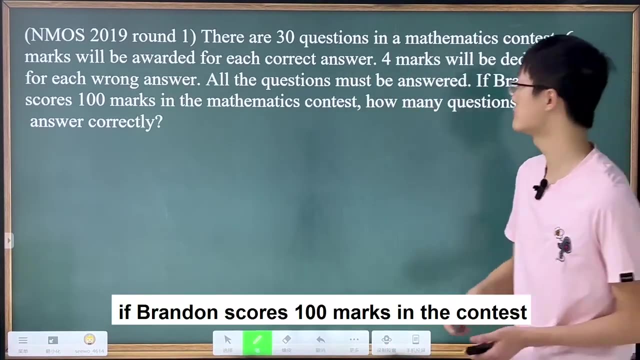 There are 60 questions in the math test. 60 marks will be awarded for each correct answer. 4 marks will be deducted. 4 marks will be deducted from the math test for each wrong answer. All the questions must be answered. If Brandon scores 100 marks in the 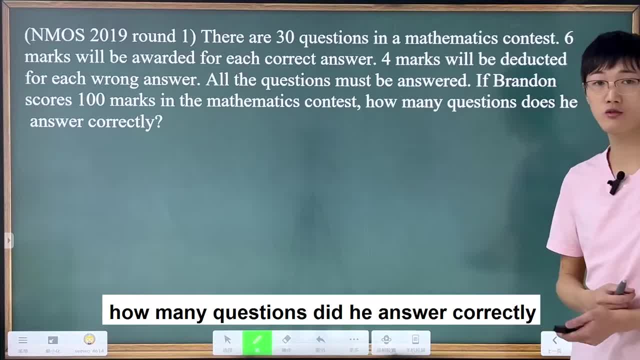 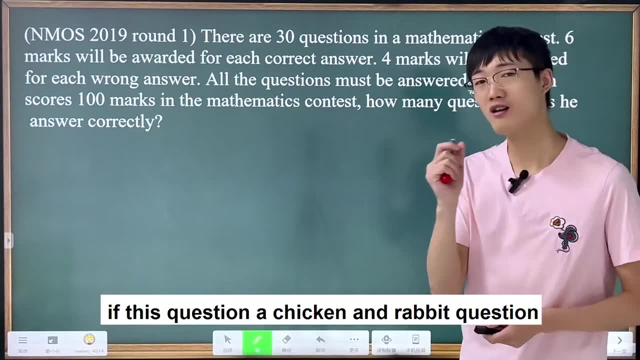 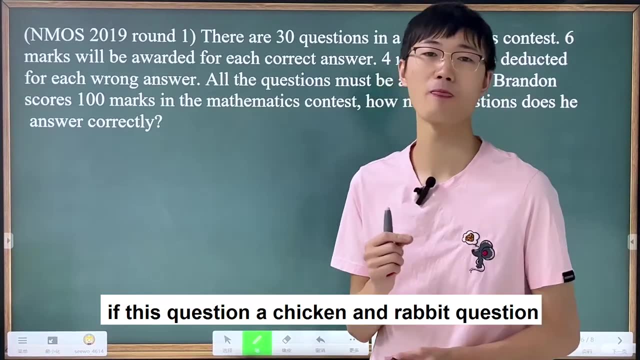 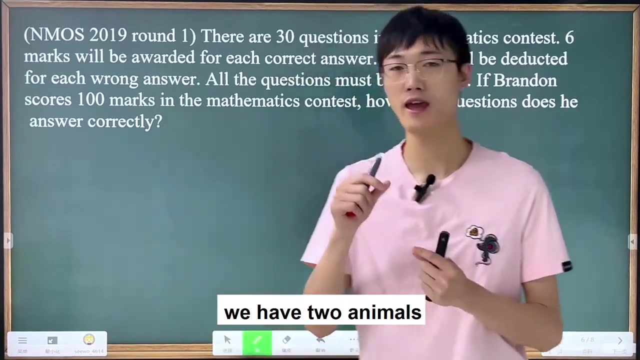 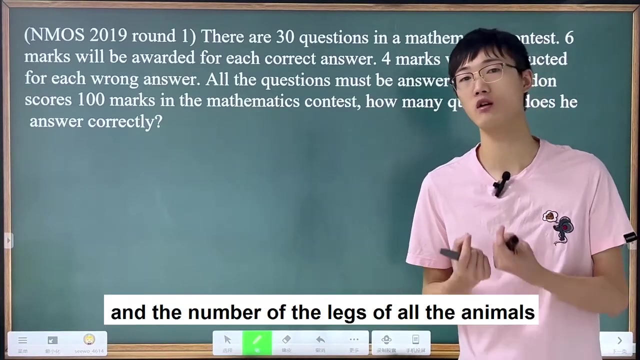 contest. how many questions did he answer correctly? Oh, some of you may wonder if this question is a chicken and a rabbit question. Think about it: In the chicken and the rabbit question we have two animals: the number of all the animals and the number of the legs of. 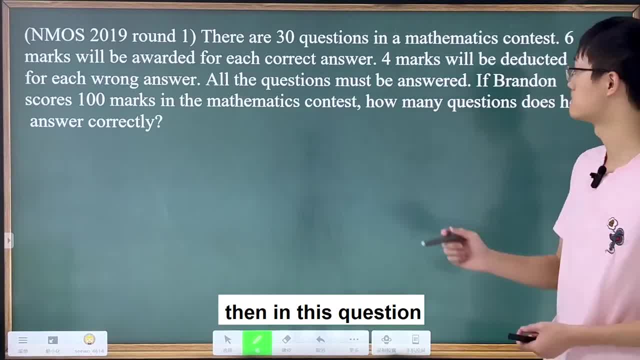 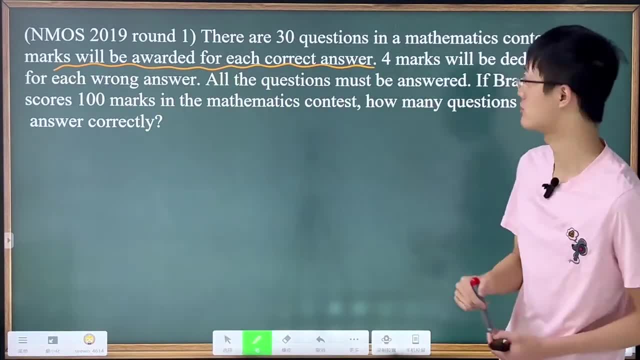 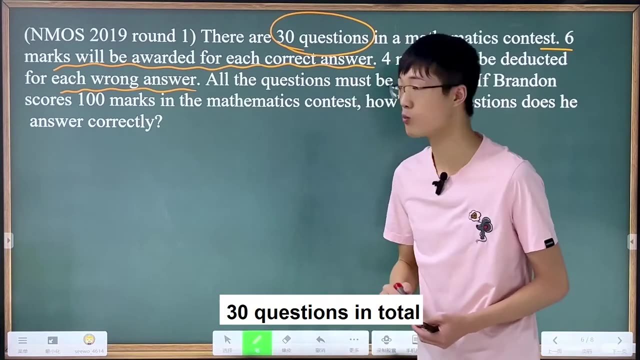 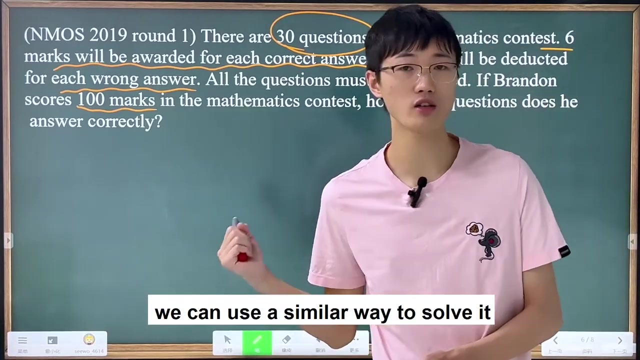 all the animals. Then in this question, six marks will be awarded for each correct answer. Four marks will be deducted for each wrong answer. 30 questions in total: 100 marks. That's very similar, So we can use a similar way to solve it. 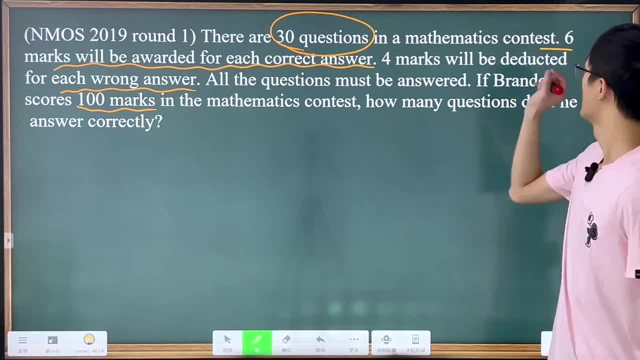 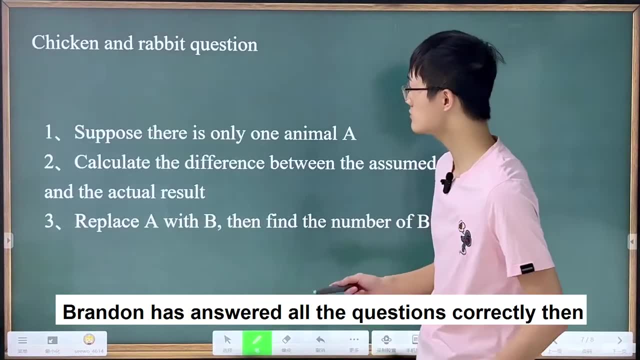 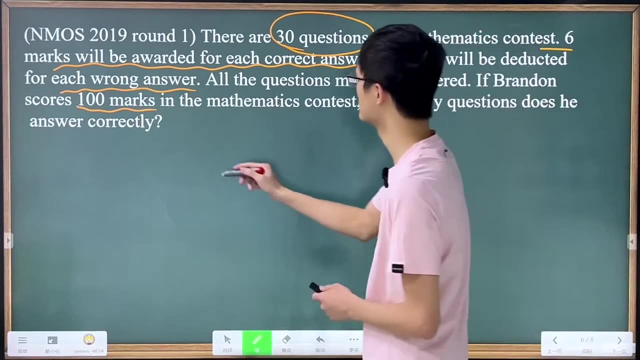 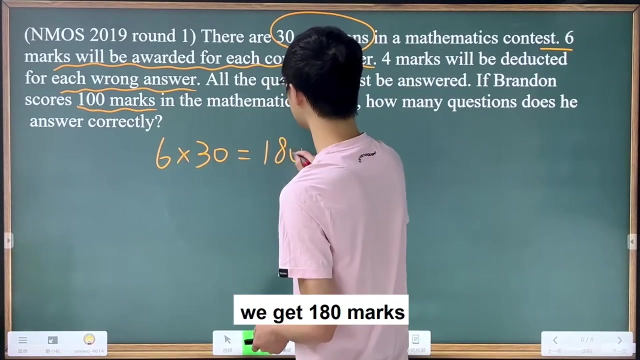 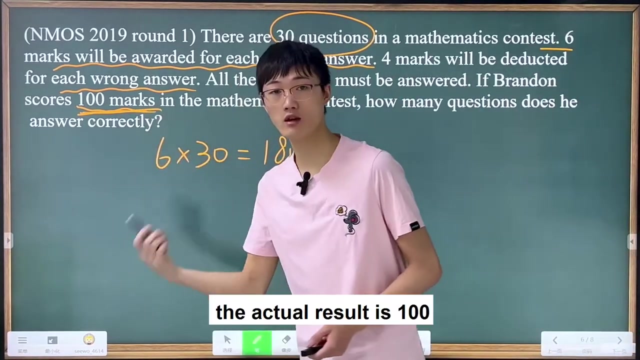 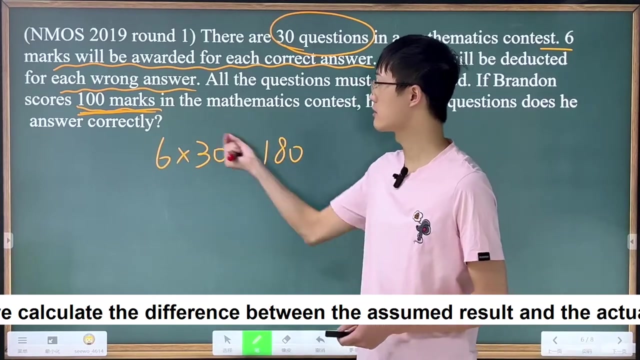 Let's go Suppose that Brandon has answered all the questions correctly, then Oh no, Then how many marks would he get Six times 30.. We get 180 marks. Then the actual result is 100.. So we calculate the difference between the assumed result and the actual result: 180. 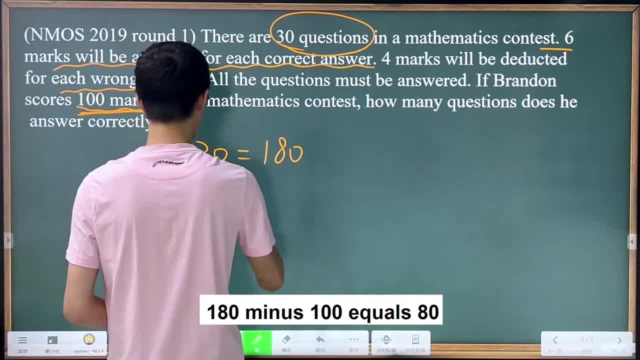 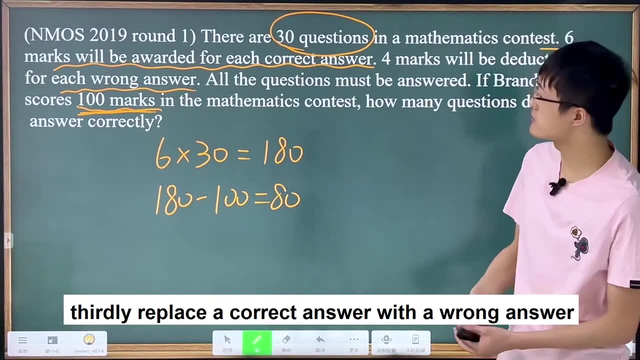 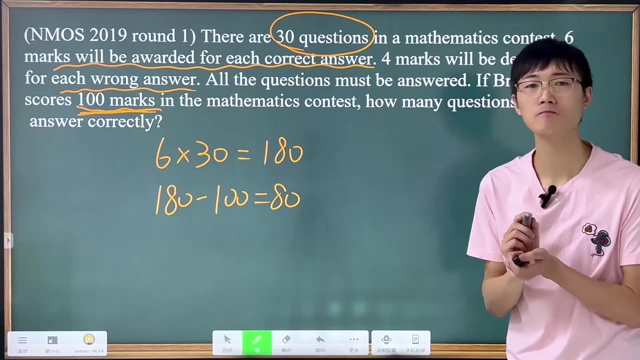 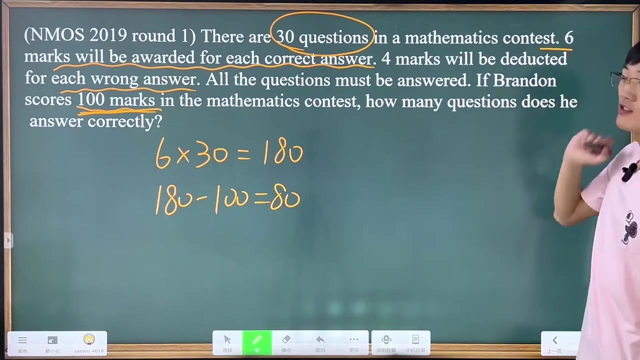 180.. minus 100 equals 80. Suddenly replace a correct answer with a wrong answer. But what will happen? That seems a little difficult. Let's see. Six marks will be awarded for each correct answer. We mark it Plus. 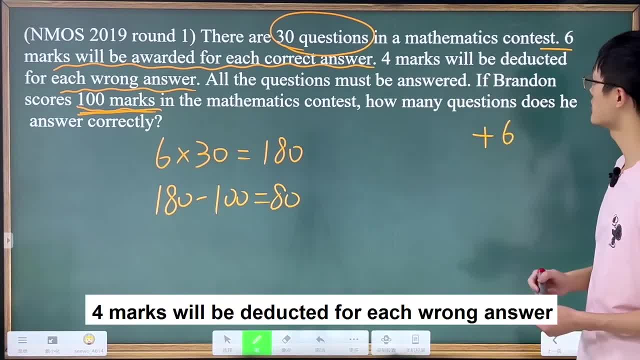 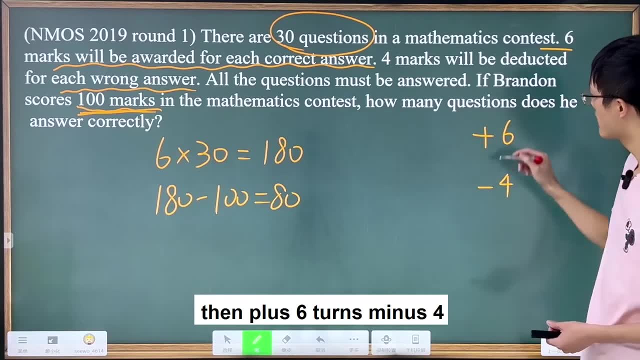 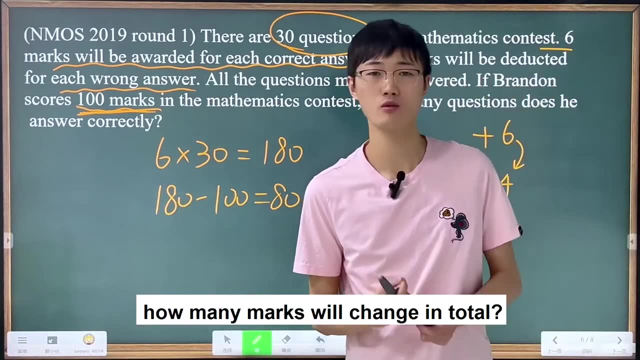 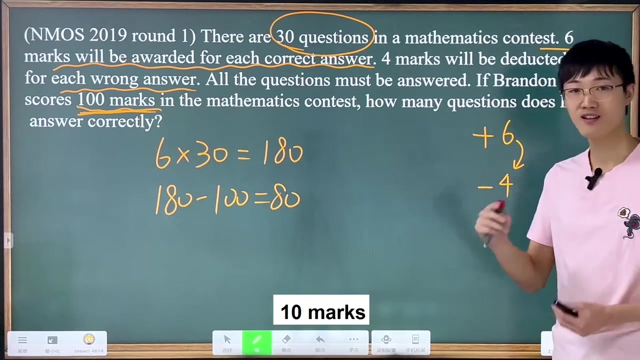 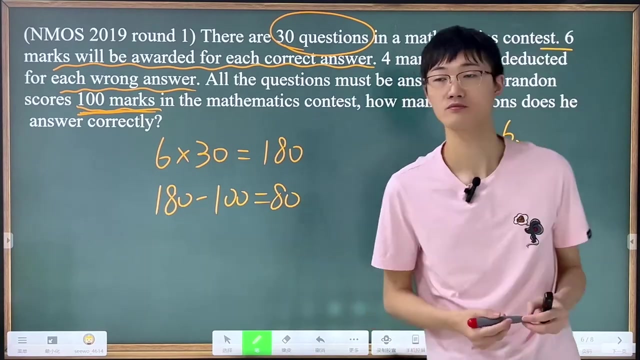 Six Four marks will be deducted for each wrong answer. We mark it Minus four, Then plus six. turns minus four. How many marks will change in total? Yes, ten marks Plus six. turns minus four: Ten marks will be changed, So our target is 80.. 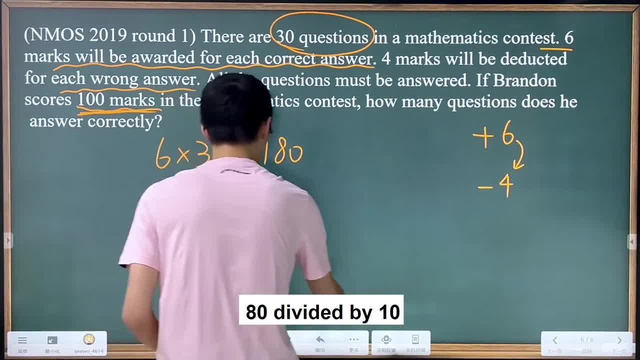 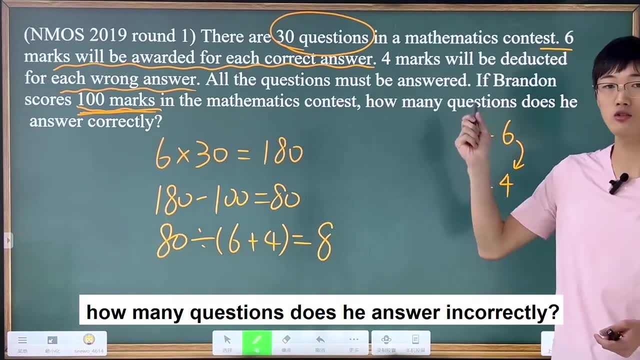 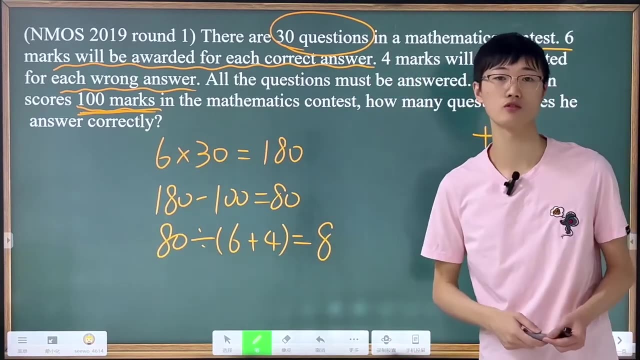 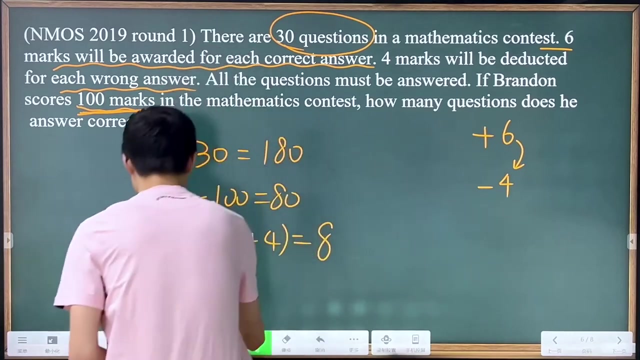 80 divided by ten, The result is eight. So how many questions does he answer incorrectly? Yes, eight questions. So how many questions did he answer correctly? Yes, eight questions. So how many questions did he answer correctly? 13, 12.